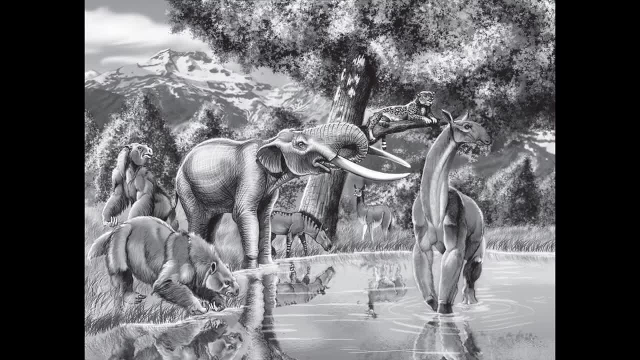 high in the food chain and they're high in the food chain. So if some small change is happening throughout environment or food chain, they'll be first to respond. Then very small populations as well. they're not sustainable and they will extinct or evolve faster. Complex communities. 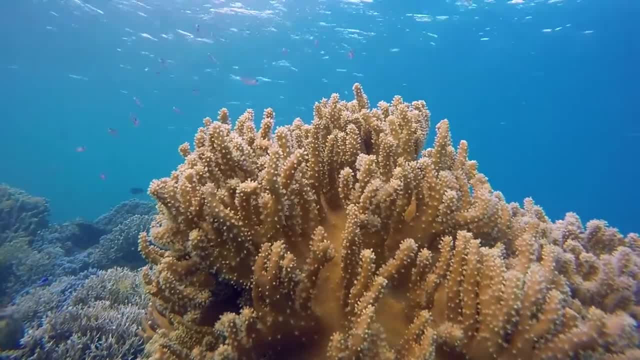 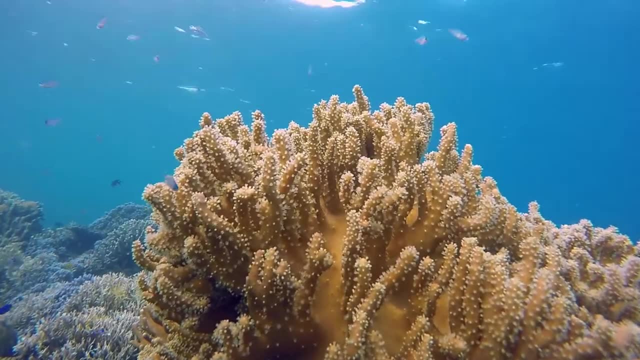 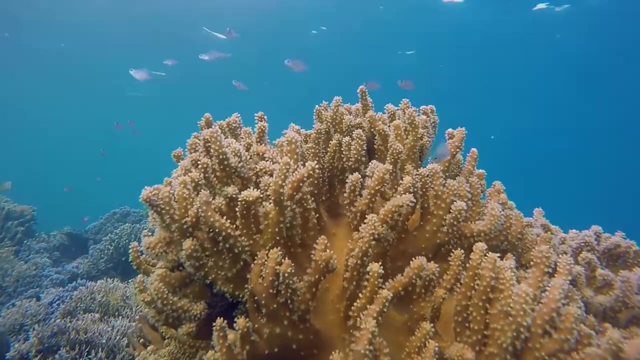 which rely on other species more prone to extinct as well, And very specialized organisms with specialized ecological requirements. So they're not very sustainable as well, And the way how they will evolve to extinct will depend on the pressure- evolutionary selection pressure- which apply to them. So it's a pressure which is applied to this community or 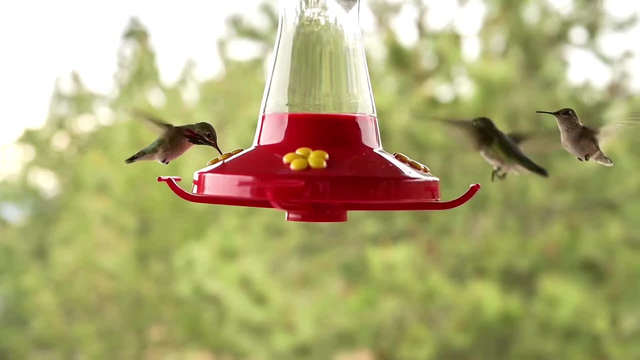 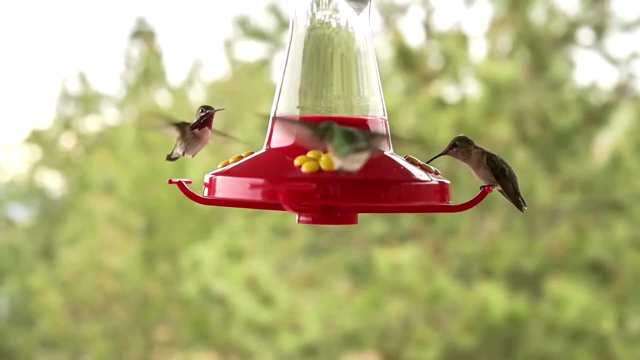 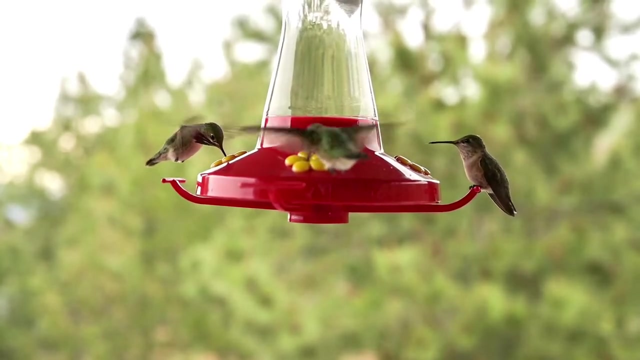 population of organisms to actually cause the change in them And they will all evolve or they will just extinct forever. We differentiate: low pressure cause just slowly, gradually change for these communities and they become long-lived And if they're not surviving that they will probably. 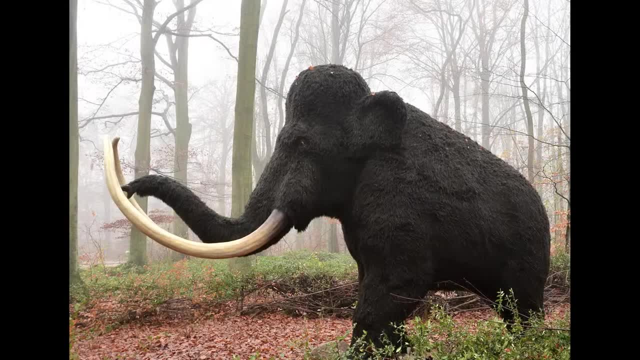 be just extinct And we have a high pressure. High pressure could be something that react very fast or very demanding. And these organisms, they don't have time to evolve or adjust to new conditions and they need to respond by extinction And often extinction happening over the evolution. 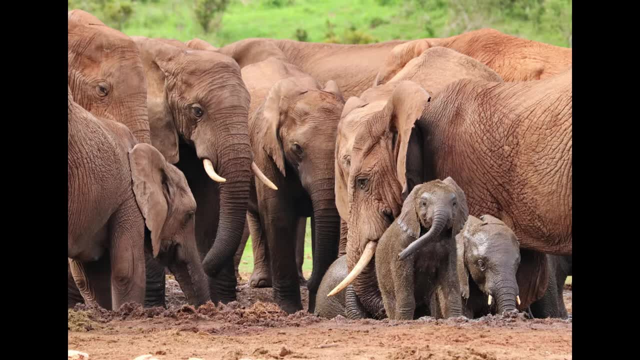 So some organisms evolving, some inevitably will die out. We differentiate different types of extinction: Internal, like predatory, and prey relationships, like growth of one population over the other and competition for space or for some food Nutrition supply. We have external type of pressure, such as environmental change. 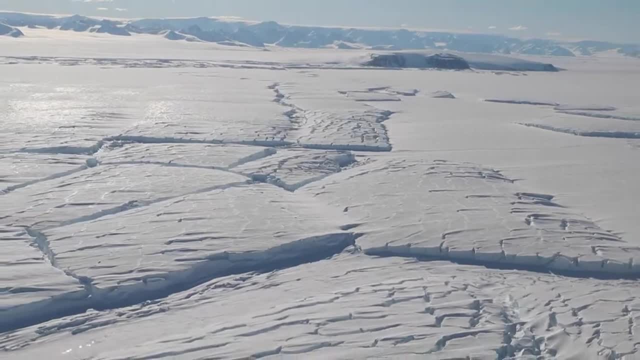 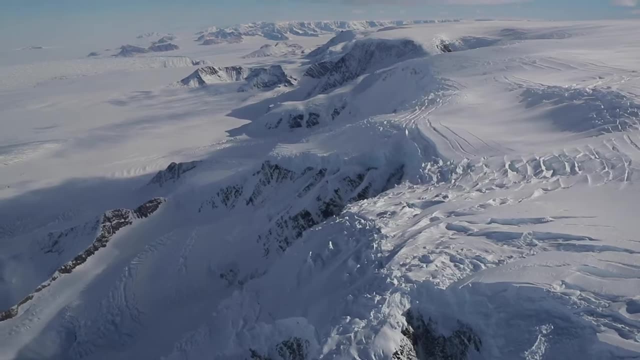 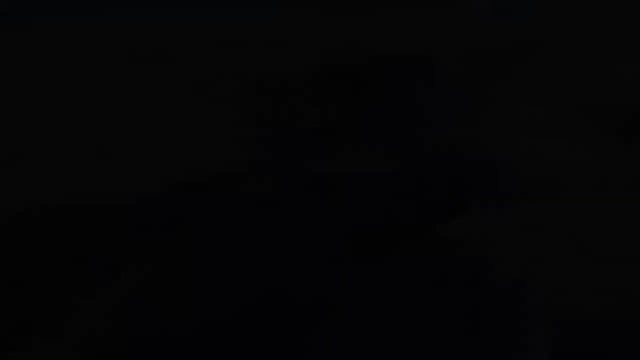 sea level change, change of composition of atmosphere or water temperature, and also change in the food supply, Nutrition, available for these organisms as well. Therefore, the extinction is inevitable. Otherwise, as I mentioned before, if all evolved organisms stay with ancient ones, the pre-ancestors, our planet will be overwhelmed with too many species. 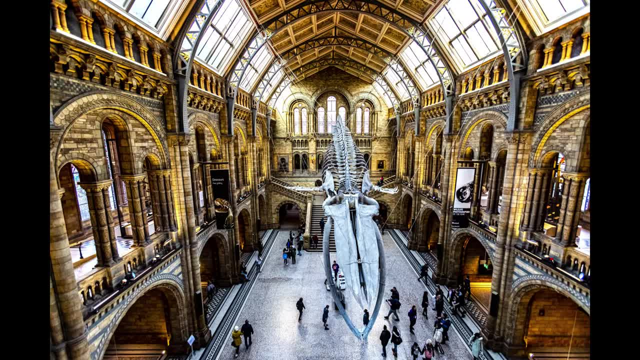 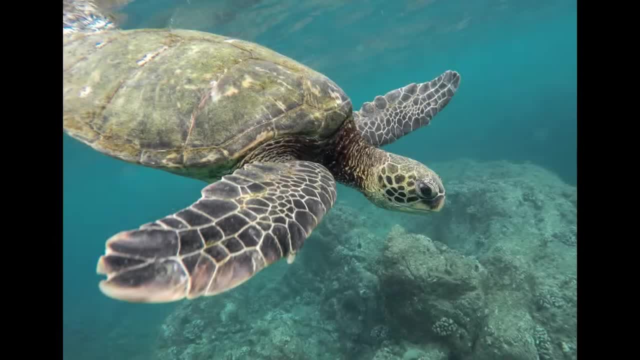 too many complex organism relationships and it won't be sustainable. We have different levels of this pressure on these organisms, So it could be just a long-term, persistent pressure which cause slow change in this species community, For example, competition between different species. We have environmental types of pressure. It's a long term, but 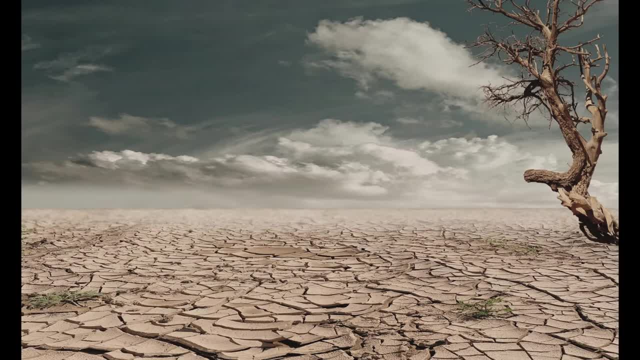 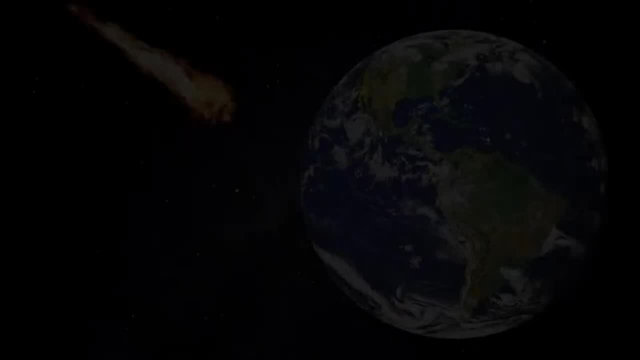 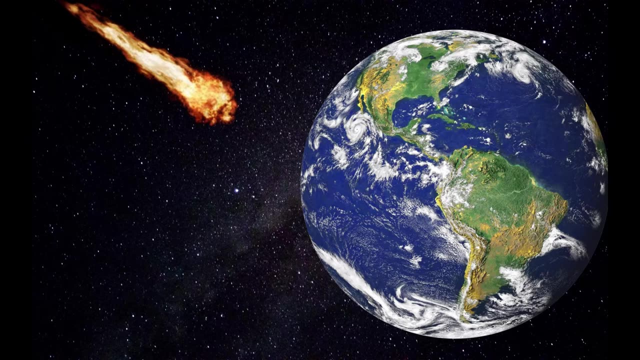 inevitably, if the environment dramatically changes, animals need to be evolved or to extinction And we have events which happen very fast and just destroying communities in the one event, such as meteorite impact or some volcanic eruptions, Meteorite impact which will dramatically 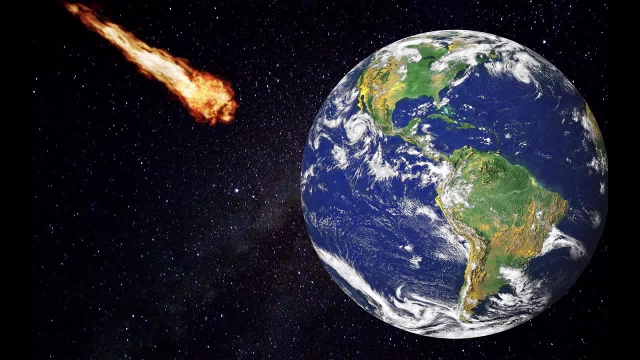 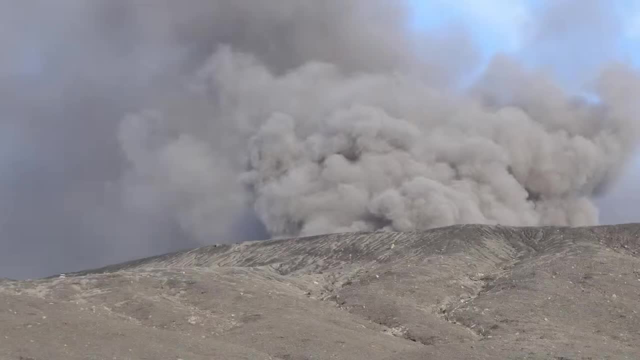 change all environments on the planet for several years and even hundreds of years or thousands of years. many species will not recover from that. With volcanic eruptions, the composition of the atmosphere change, AND SO ON, It can be aluded- environment also made of even more than several. 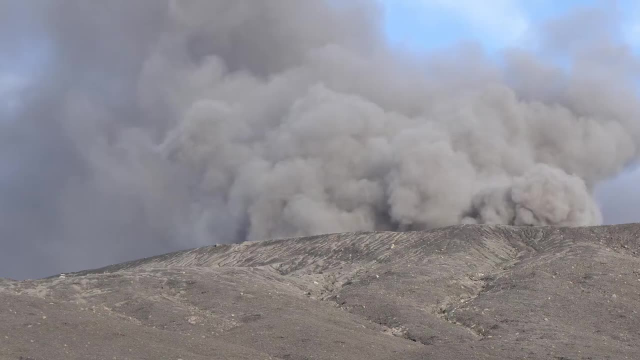 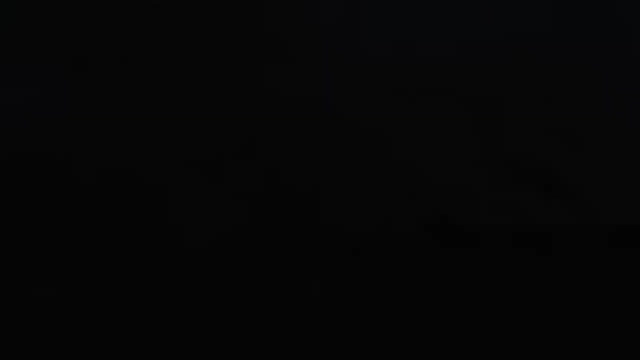 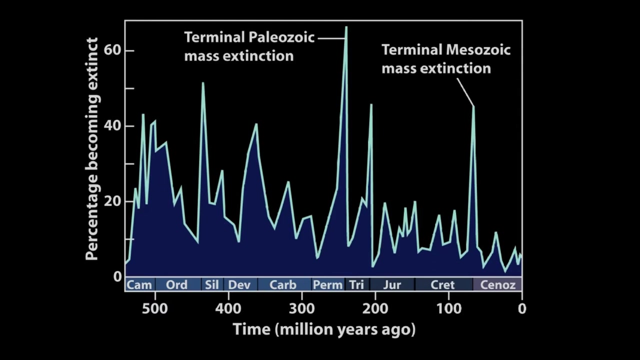 changes. there's a lot of serum, carbon dioxide explosion into the atmosphere and not all species will survive after that. when we look on our time table, we see that in last 450 million years we have spikes of dramatic extinction. this graph shows the number of extinct species throughout. 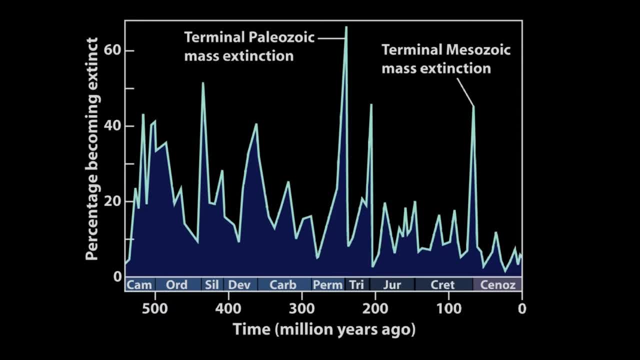 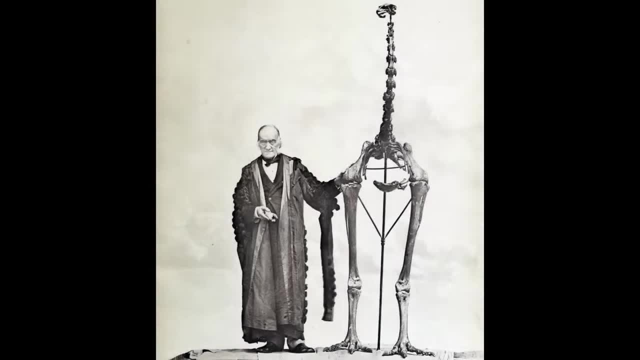 the history of times and of course there are some animals we can observe who extinct, like, for example, in recent human history. there's a lot of animals extinct, like more birds in new zealand and we know they were there, we observed them and now they've just extinct. but there's also 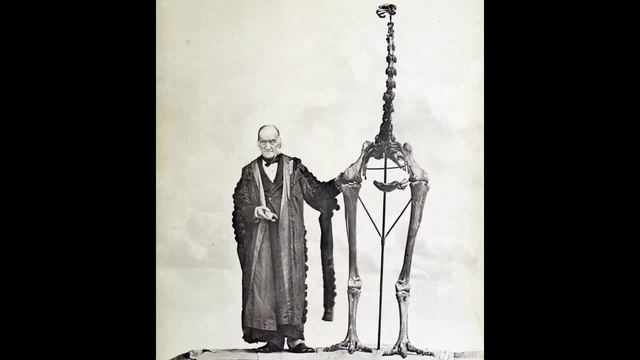 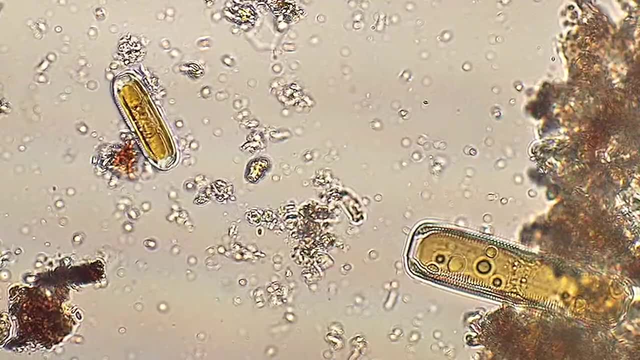 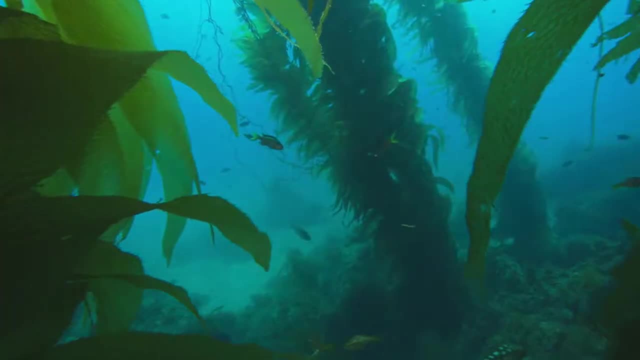 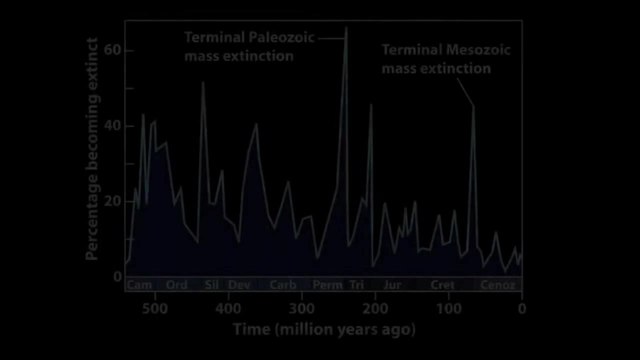 numerous animals which we're not aware are extinct and they doing so every day: instincts, attack of small organisms, type of sea organisms which we don't see and we don't think this happening with them. but the extinction happened in our planet all the time as, especially since the humans affecting the environment very fast, in the history of the 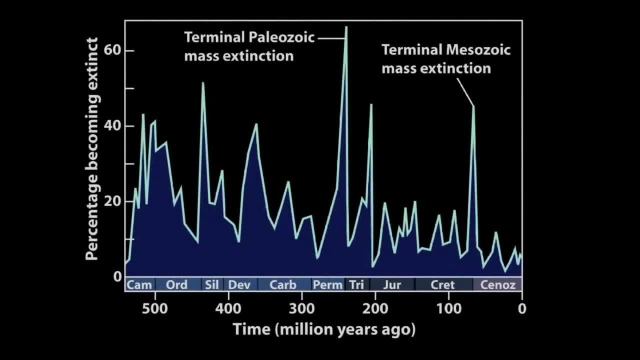 earth. usually, this extinct event will be related to environmental changes or some dramatic events like meteorite impact, for example. if we looked on famous or the weak extinction which happened about 440 million years ago, it was time. what's happened- great cooling on our planet. we're not. 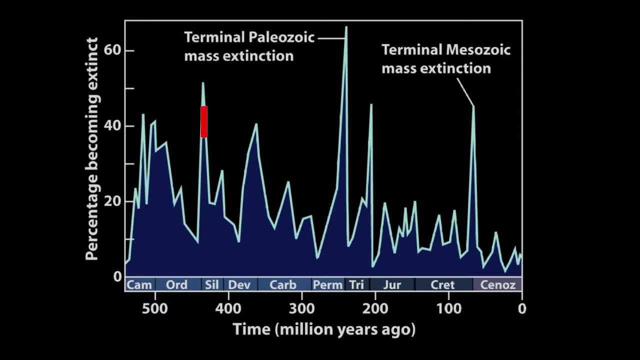 going to talk about the reasons why there's many conspiracies and theories why this cooling event happened, but we definitely know that planet was warm before there was no ice in the poles. the ocean was circulating in the way that it's redistribute the heat equally everywhere and 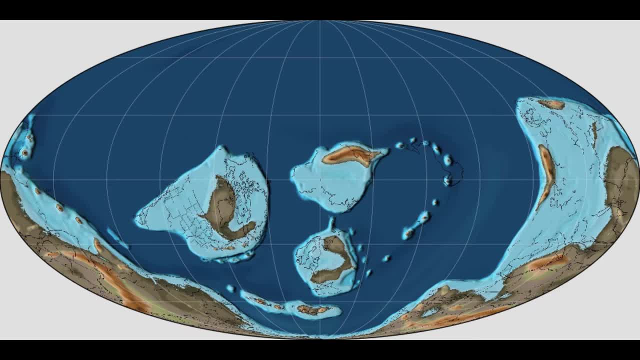 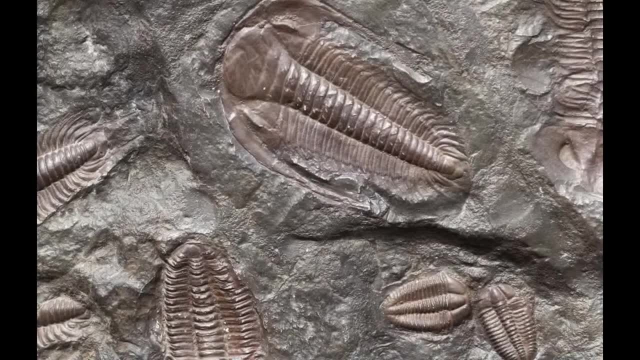 there was a very nice and good condition for life to strive. then something happened and cooling event changed the ocean work and extinction followed. drop of sea level and this cooling event caused extinction for almost 85 percent of species who was on the planet at the time. according to scientists, however, the planet recovered from that. there was a long term of 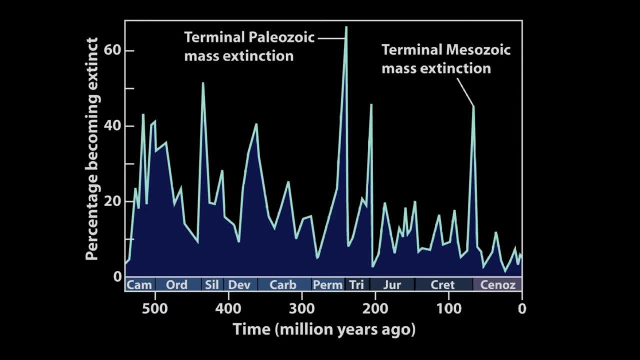 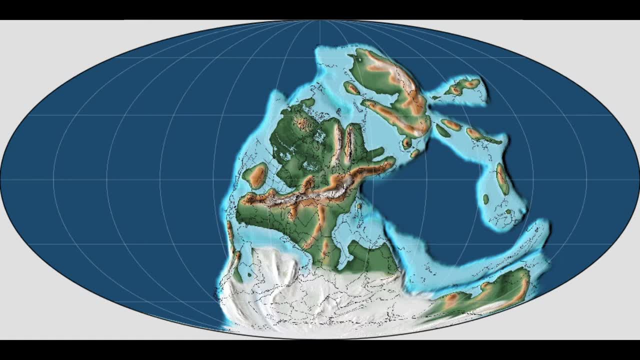 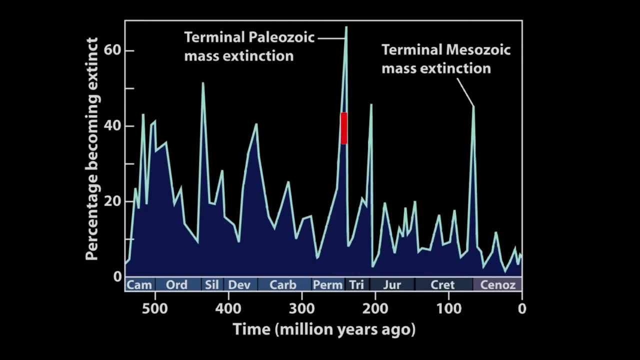 about 100 million years of more warmer periods and ecosystems become more stable again, and it was a pretty good time for them to live on our planet until next big event, which was rapid increase of the temperature on the planet in the permian time, which caused another extinction event. 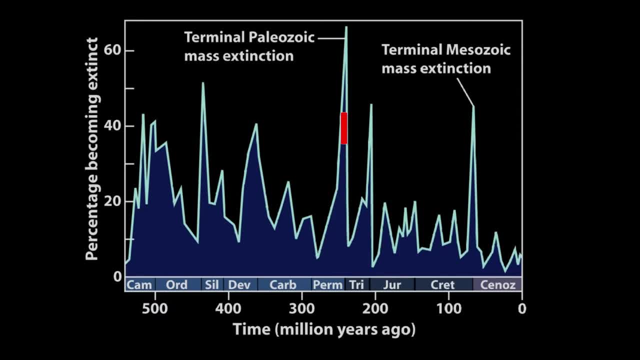 it was the biggest extinction. there was a too dramatic increase in the temperature on a planet, a change of climate, and animals couldn't adapt as fast and we lost about 96 species on the whole planet, 65 families. after that you can see that there was a gradual recovery, with some smaller. 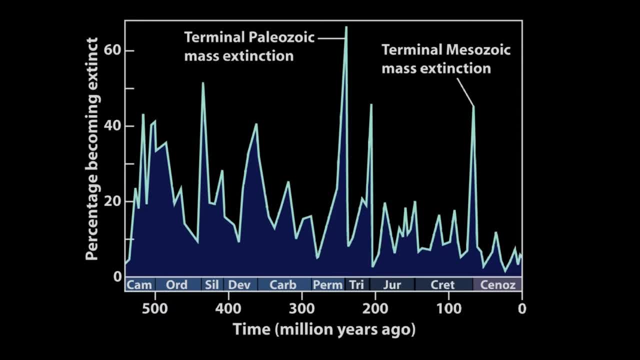 extinctions on the way, but animals had fairly warm climate and mesozoic times and the evolution spiked their time, of course. so you can see permian extinction was the biggest so far on our planet in the history of the animals. and before that we have long time when the environment was fairly 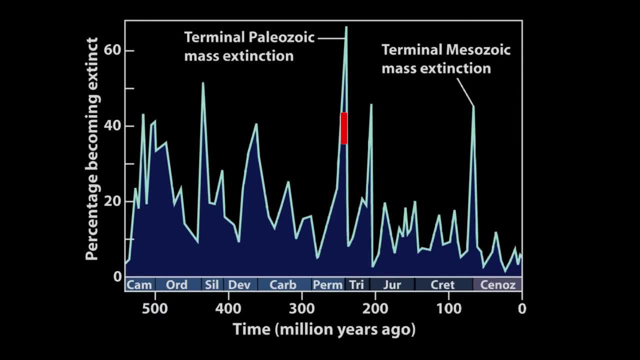 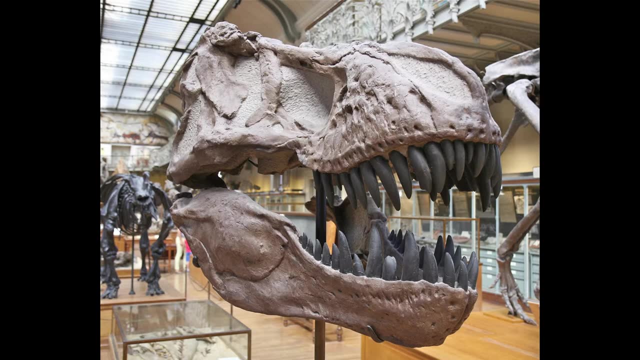 stable and the animals have time to evolve and live for longer times. after the permanent extinction, again when the environment stabilized, organisms had opportunity to recover and slowly evolving in the not so much dramatically changed environment. mesozoic time famous for reptile strive on our planet and you know it by 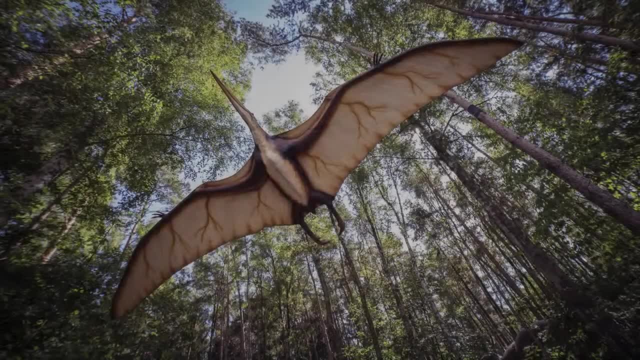 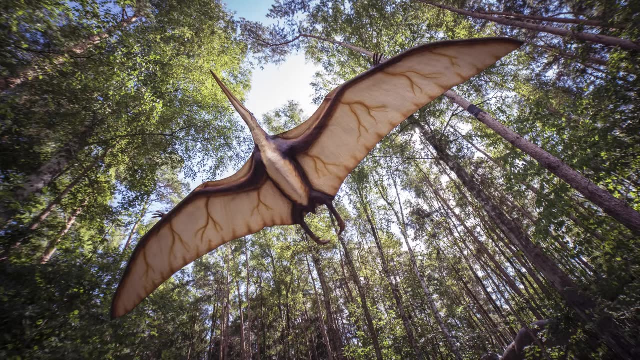 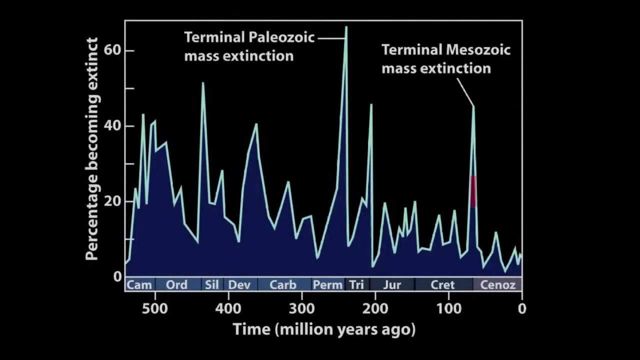 all famous dinosaurs developing on our planet and also of beginner of the birds age. then we have the terminal mass extinction in mesozoic time, 66 million years ago, one of the most dramatic extinction we know about, when all the dinosaurs die out on our planet and scientists convinced that it wasn't environmental change as much. 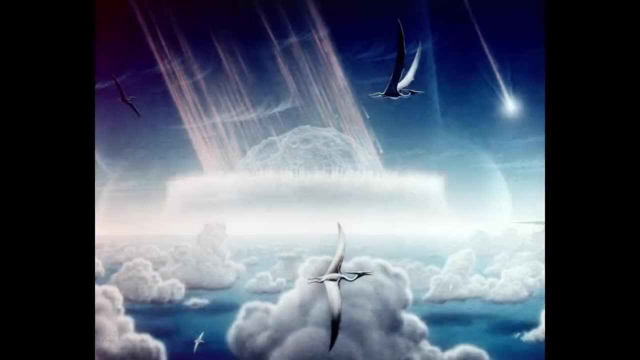 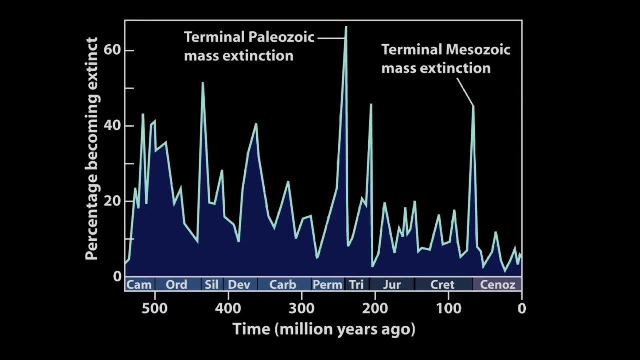 that it was a meteorite impact. it was a dramatic event. we see all around the planet in geological record and its abrupt event, which caused extinction of most of the reptiles on our planet. since then we had fairly warm period of time. evolution take place and only last 20 million years. 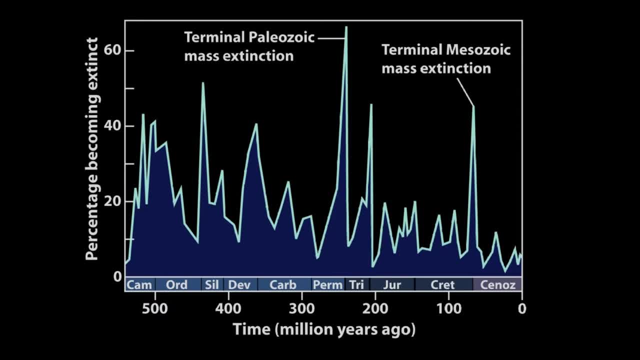 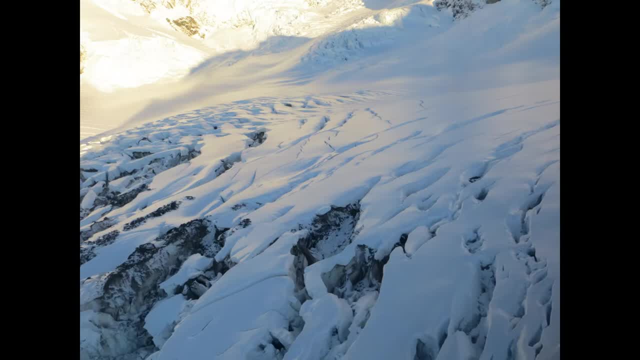 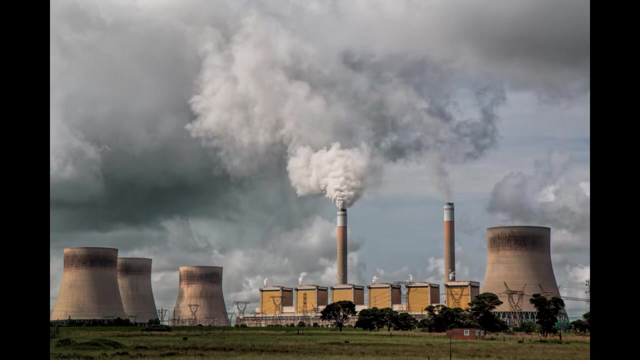 we have colder climate on the planet. when ice ages come in place, we start having ice everywhere and in the blink of the history of the planet, humans came. and the moment when humans came, scientists suggesting the biggest mass extinction right now on our planet happening by impact of us. in the future we'll see the effect of last. 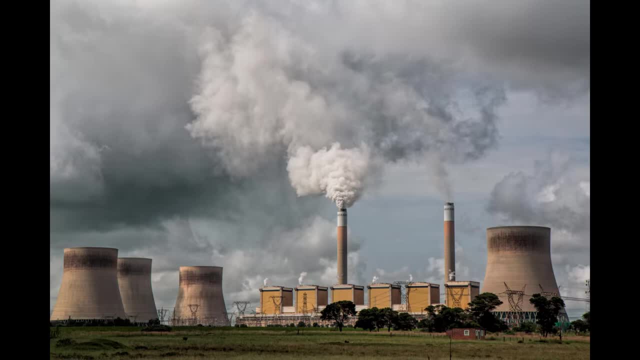 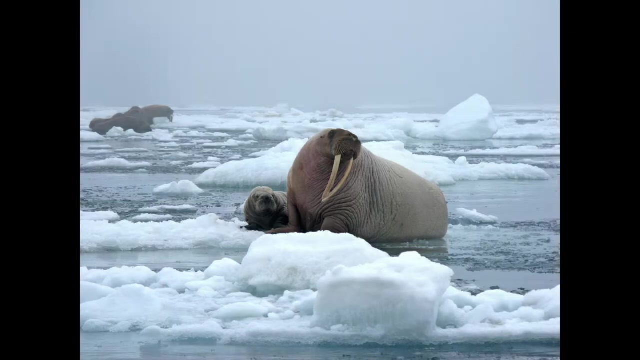 mass extinction which is happening right now on our planet, and the main question remained if the ecosystem will have time to adopt or will lose many families forever. however, it's the first time in the history of the planet there's a too short time for animals to evolve and adapt for very rapidly changed environment due to the human activity. 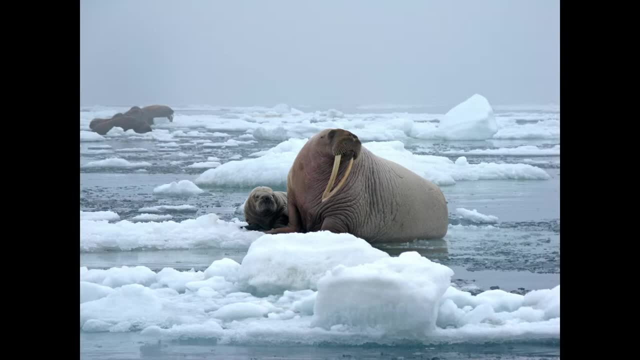 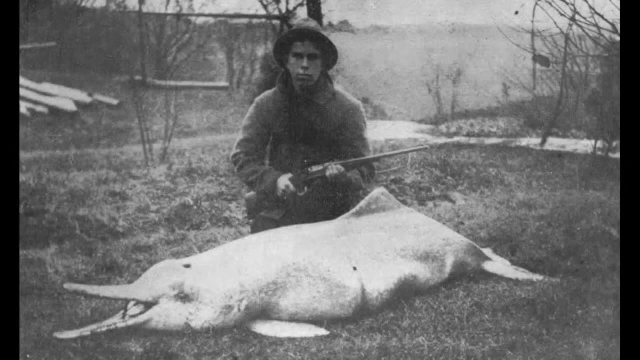 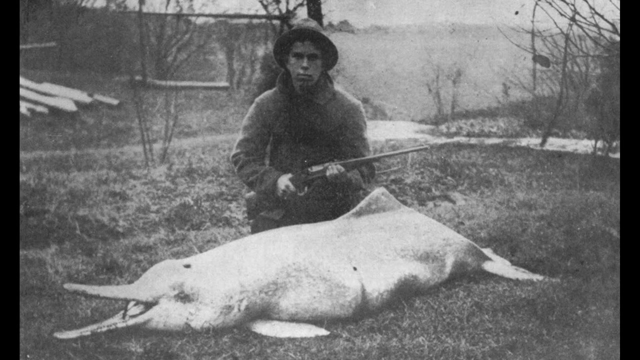 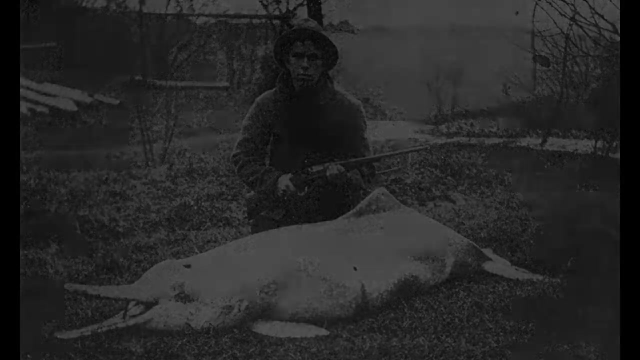 therefore, we might lose forever many families in species on our planet, like already happening these days. for example, chinese dolphin will last seen in 2007. it was the last animal of the species which died. therefore, our children will never see alive this animal anymore, but the history show us that animal world will evolve no matter what a catastrophe happening on. 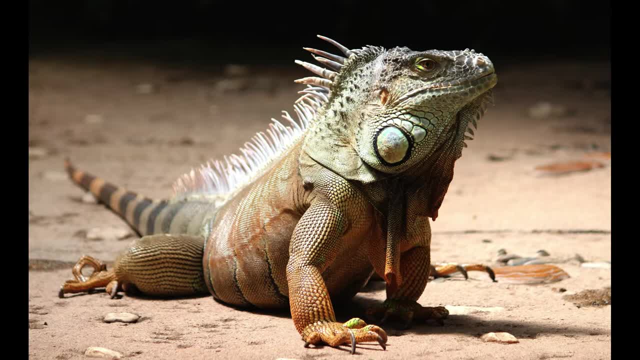 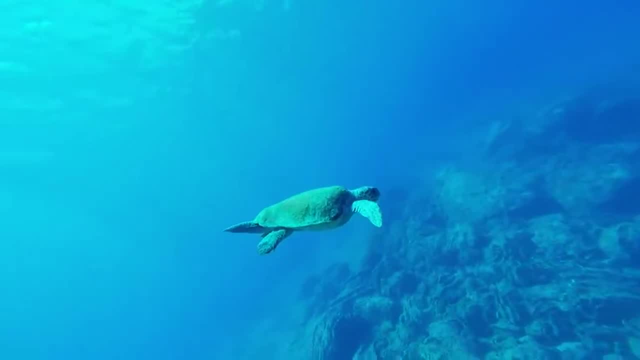 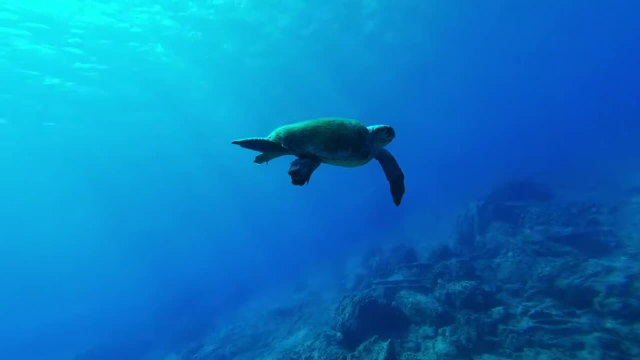 this planet. therefore, like since meteorite killed most of the reptiles on our planet or dramatic climate change in permanent time caused almost full extinction of animals on the planet, in the many thousands and millions of years the new types of animals will evolve and occupied our planet all over again. 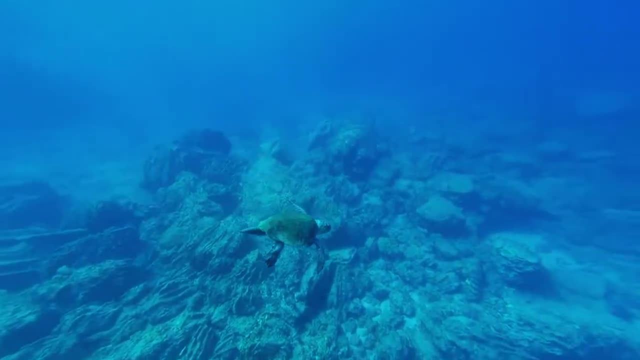 so in the end of the world, we will be living in the same place as a new species. so it's a really interesting answer, and i hope that this video will help you to do the same. if you have any questions, let us know in the comments section below. or if you have any questions, please leave a comment below. we will share the information with you as much as we can, and we will see you next week.